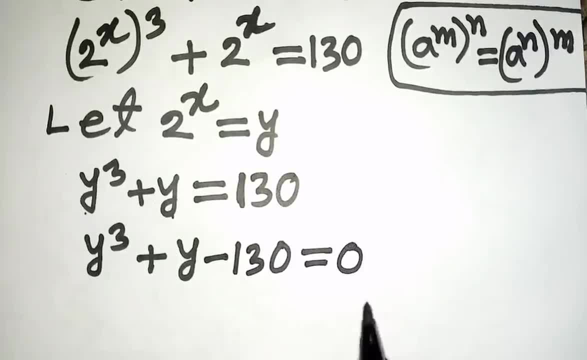 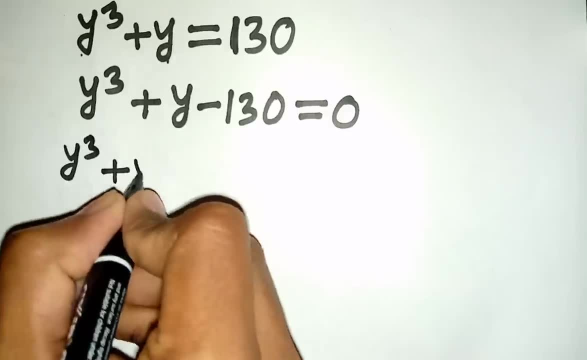 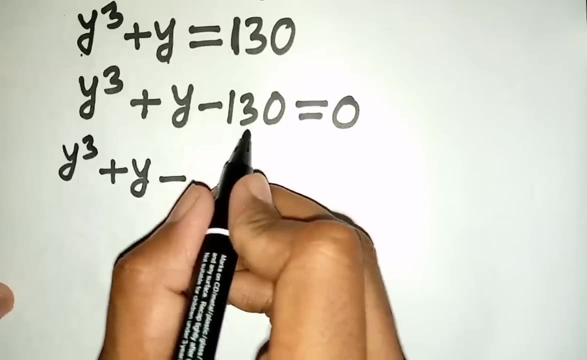 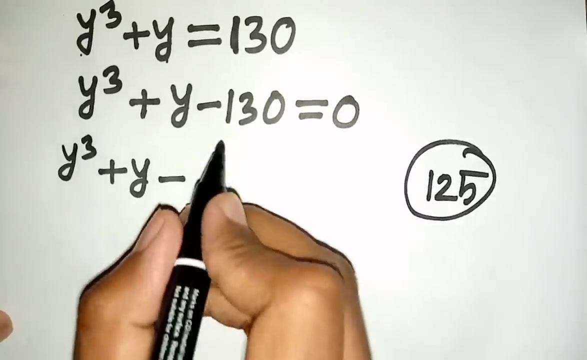 minus 130 is equal to 0.. Now we can write here: y cube plus y, then minus 130.. Attention: here cubic number of 130 is 125.. I repeat that the nearest cubic number of 130 is 125.. So 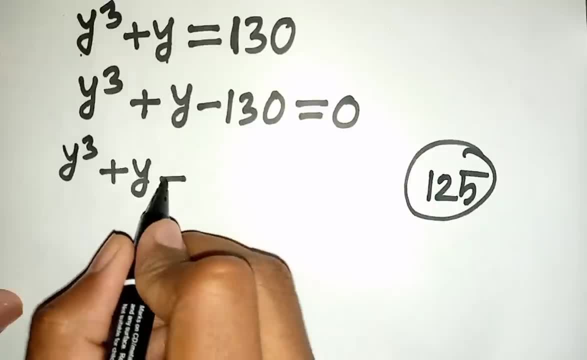 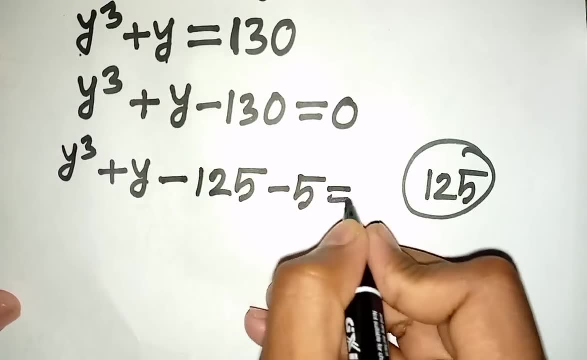 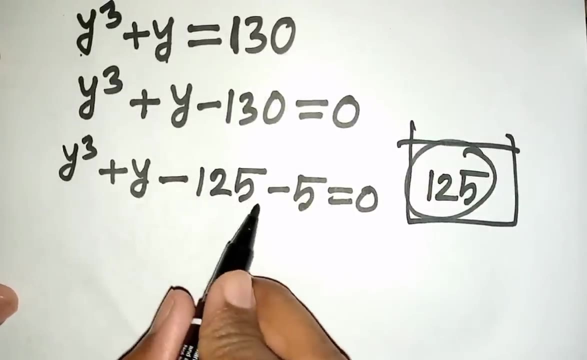 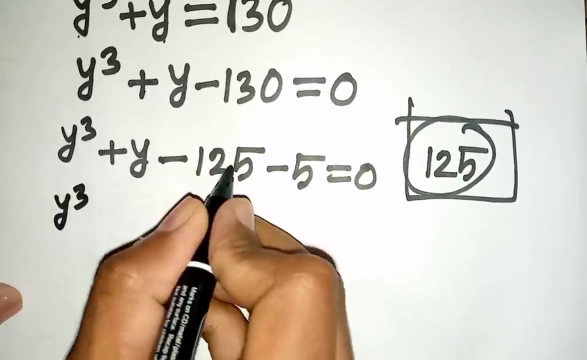 we can write here: minus 130 is same as minus 125, minus 5 is equal to 0. That means minus 130 is same as minus 125, minus 5 is equal to 0.. Now we can write here: y cube minus 125. 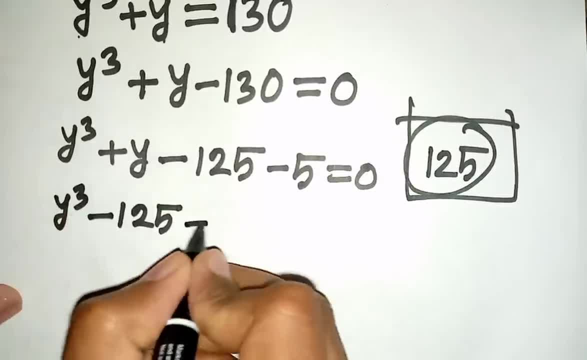 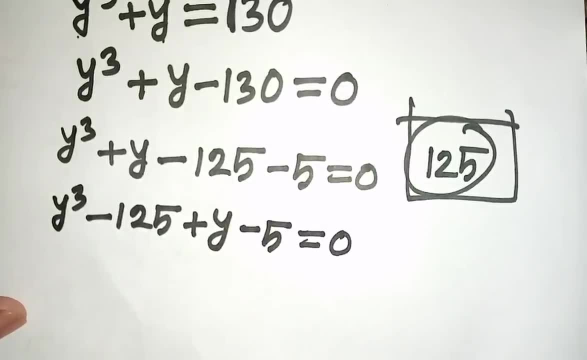 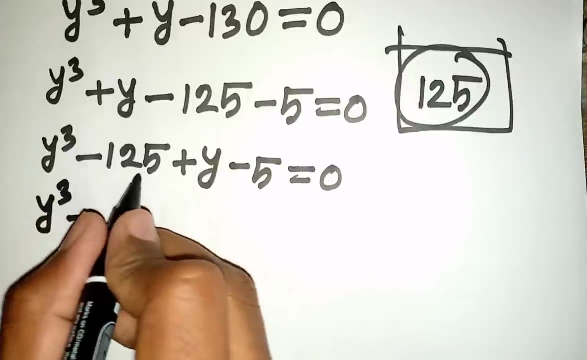 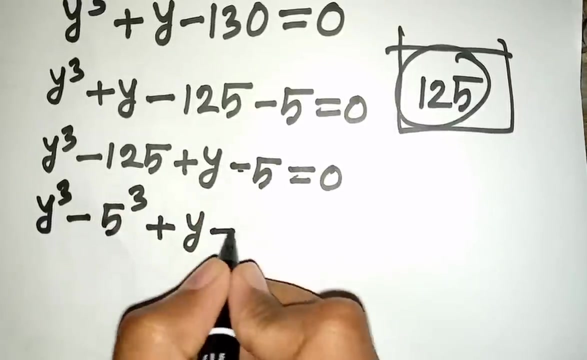 plus y, then minus 5 is equal to 0.. Now we can write here: y cube minus 125 is same as 5.. Now we can write here: y cube minus 125 plus y minus 5 is equal to 0.. Now, here we can apply. 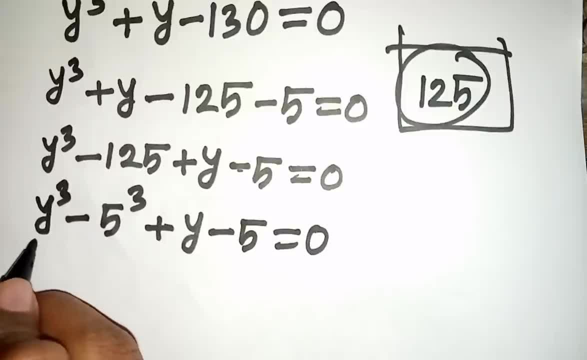 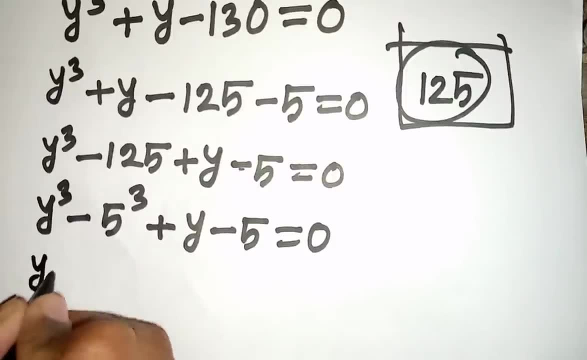 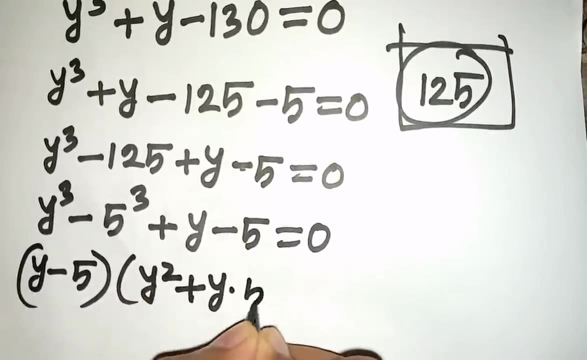 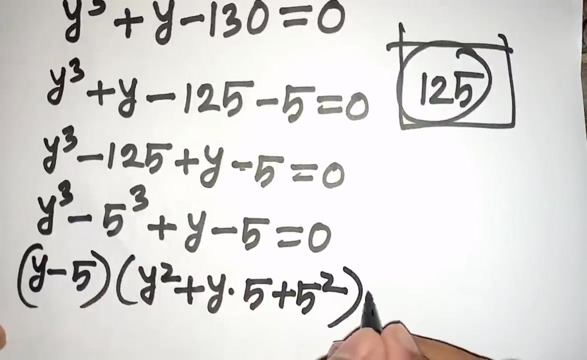 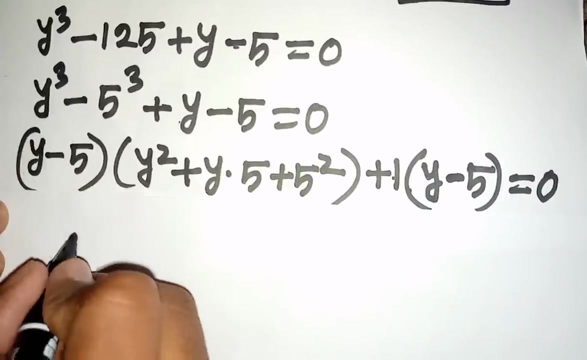 the formula of a cube minus b cube: Here a is sy, b is s5.. So according to formula we can write here: y minus 5 times y square plus y times 5 plus 5 times y square plus y times 5, by: 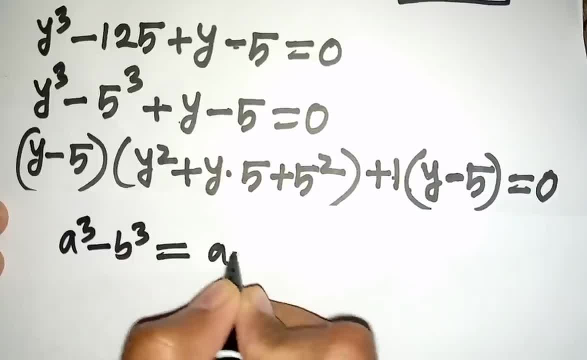 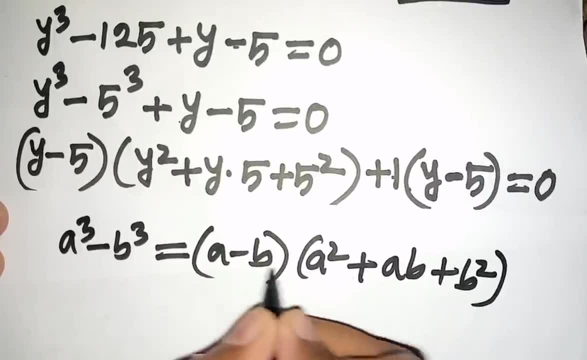 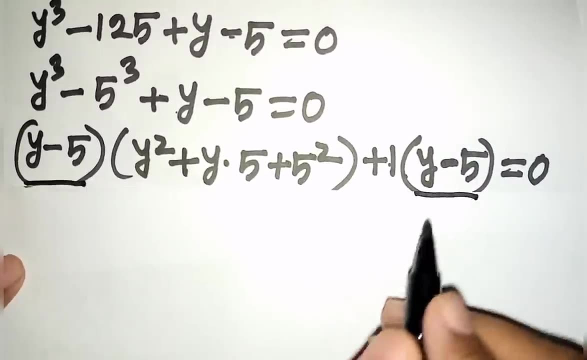 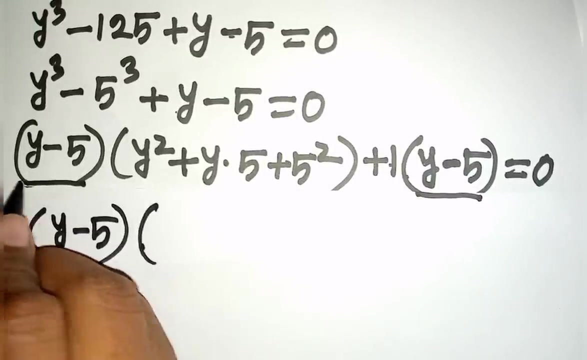 this that means y. then minus to a minus b, times a square plus a, b plus b square. now the y minus 5, y minus 5 is common, so bracket y minus 5 is out of this bracket. so this divided by this, that means y square. 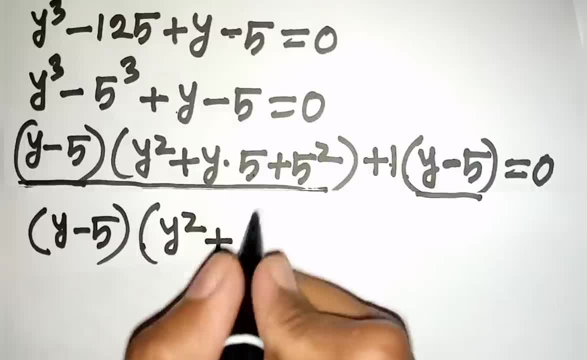 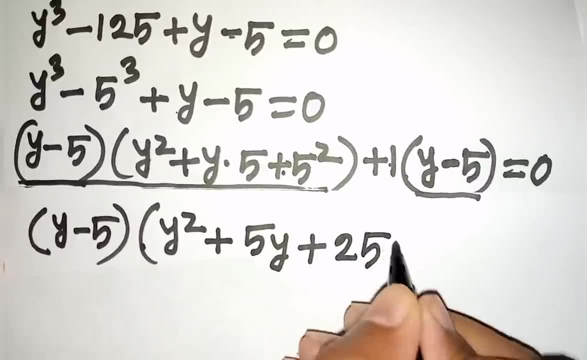 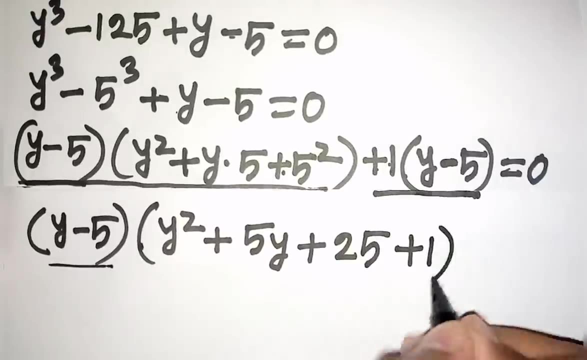 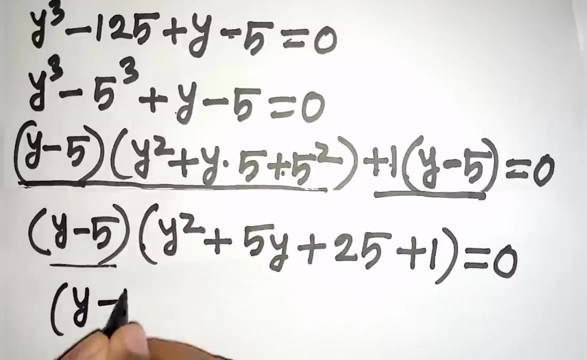 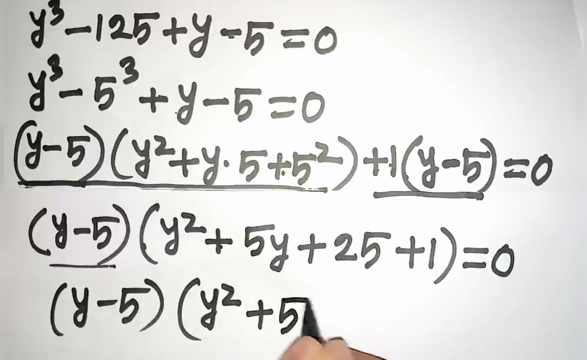 plus y times 5, it will be 5 y plus 5 square, that means 25. then plus this divided by this, that means 1 is equal to 0. now we can write here bracket: y minus 5 times y square plus 5: 5 y then plus 25 plus 1, that means plus 26 is equal to 0. now we can write here: y minus 5. 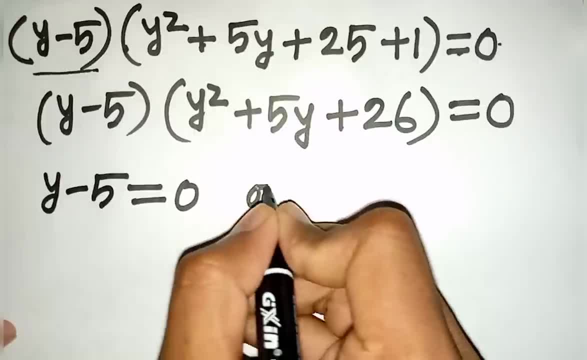 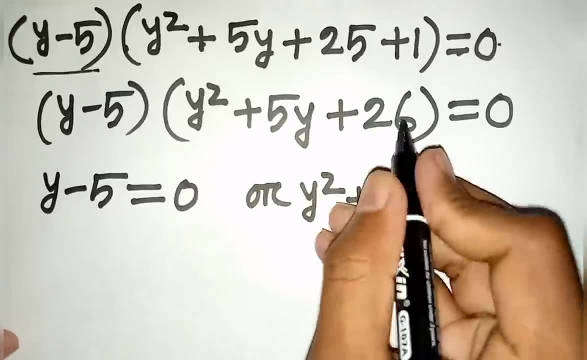 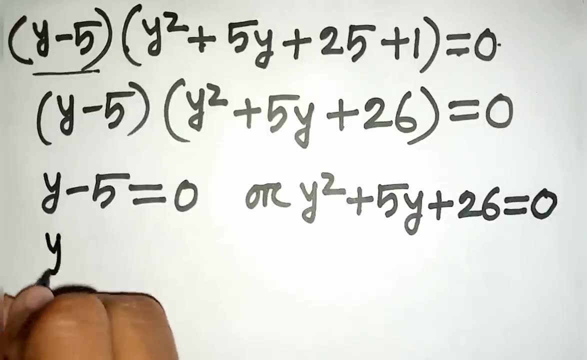 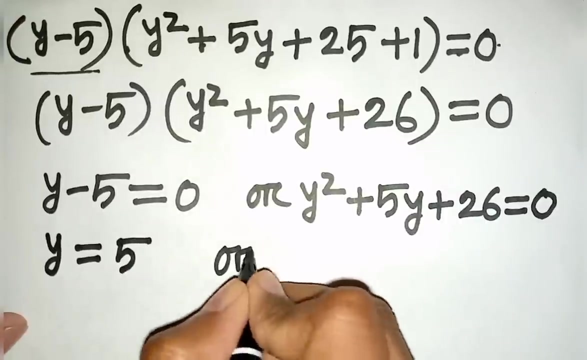 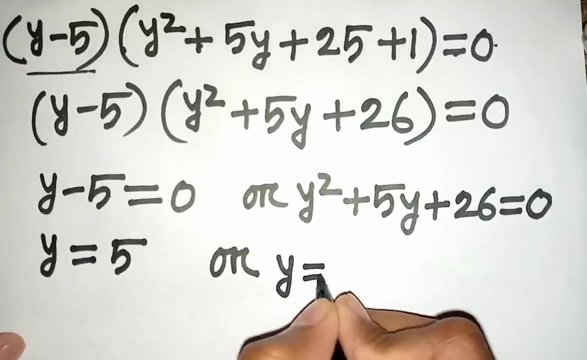 is equal to 0, or y square plus 5. y plus 26 is equal to 0. now we can write here: y is equal to minus 5. take to the right side, so this will be plus 5. or now here we can apply quadratic formula. so we can write here: y is equal to minus b. 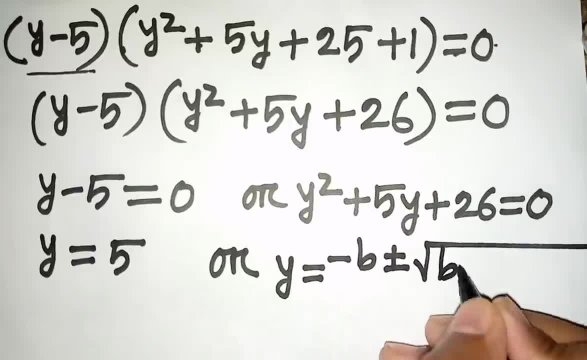 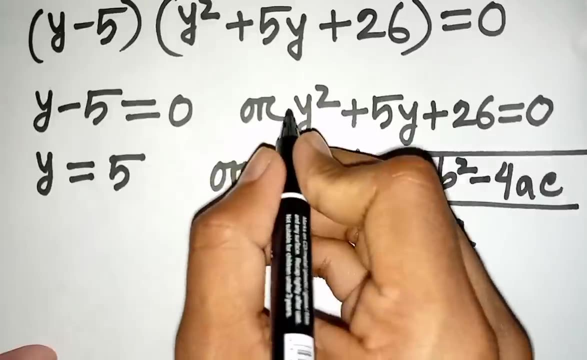 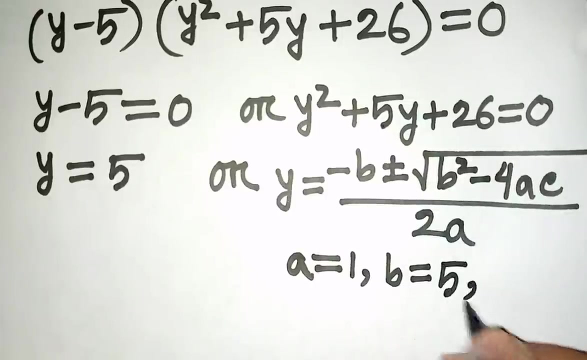 plus or minus a square root of b square minus 4 ac, divided by 2a. now here a, a is s 1, b is s 5, c is s 26. so we can write here: y is equal to minus b, that means 5. 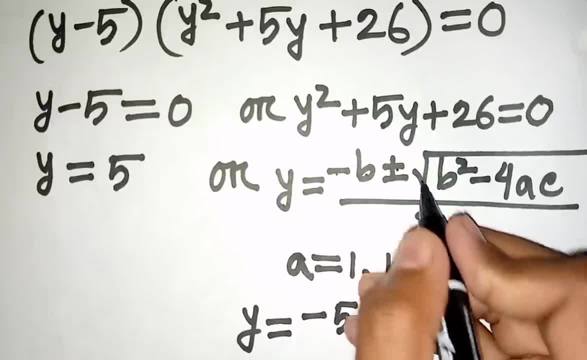 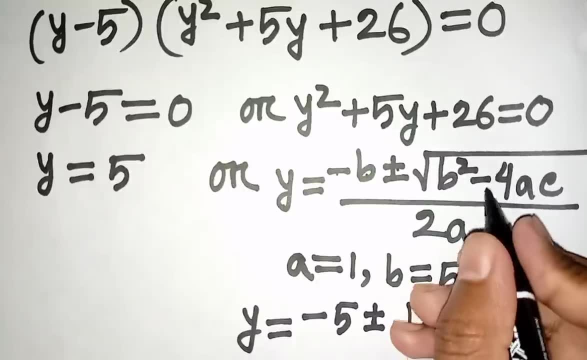 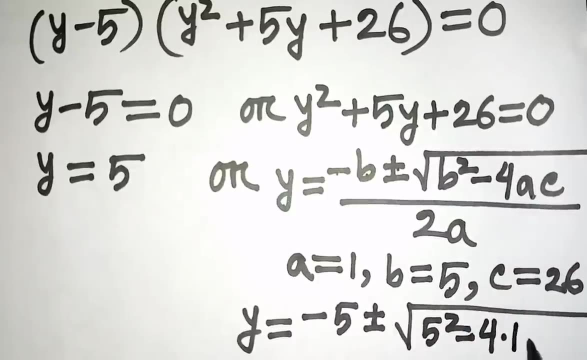 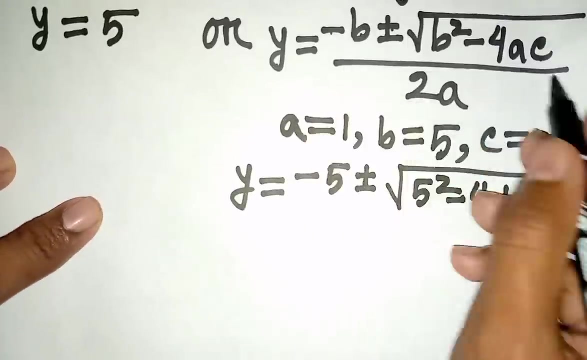 plus or minus a square root of b square. that means 5 square minus 4 times a. that means on times c, that means 26 now divided by divided by 2 times a. that means 26 now divided by divided by 2 times a. that means 26. 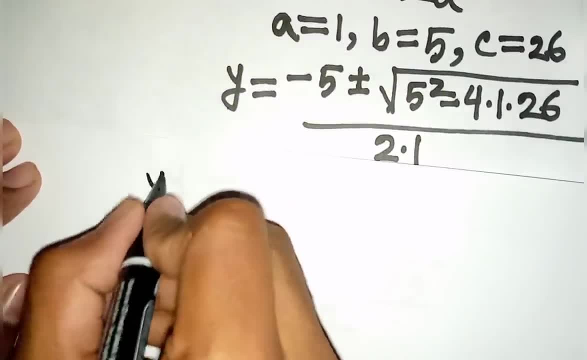 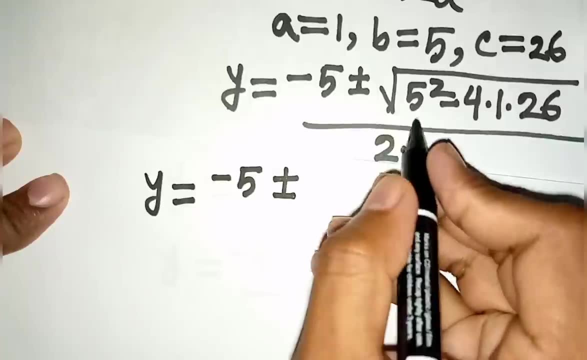 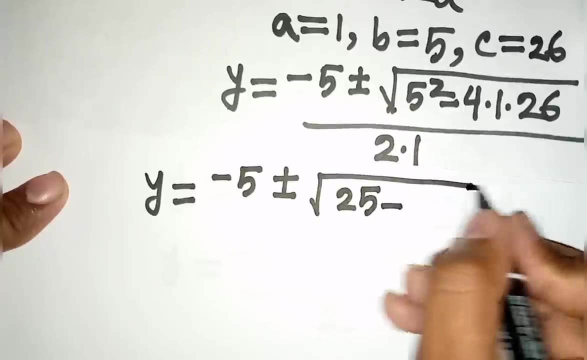 now we can write here: y is equal to 1. what is S? that means it is 0 and that means a, that means 1. that means y is equal to minus 5, plus or minus a square root of 5 square. that means 25. 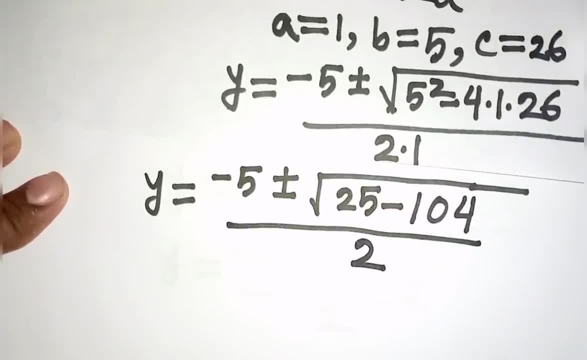 minus 4 times 1 times 26. minus 4 times 1 times 26, that means 104. divided by two times on, that means two. now we can write here: Ni twice minus a, that means 1 in case one as greater than minus 5, right. 65 minus 1 times 1 times x. this means 1 in the same structure: x. click on to the left side. that means seventy- 먼저加机. we can write here: y equals times of times 10 goes to the right hand side. 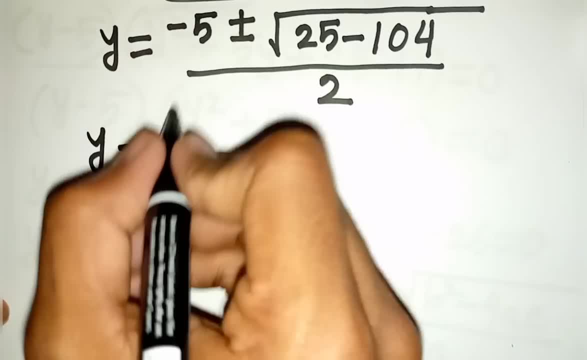 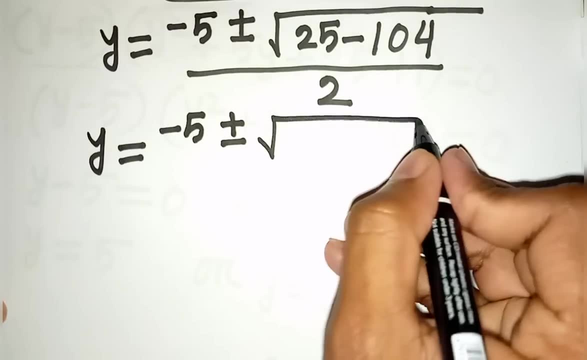 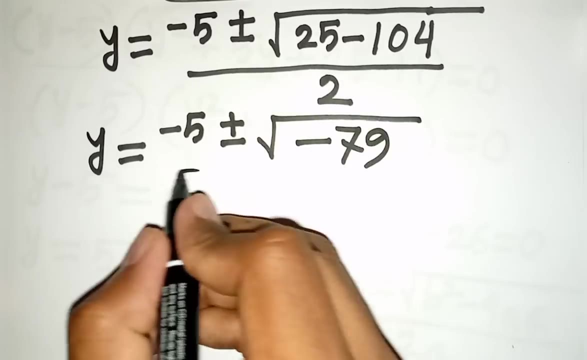 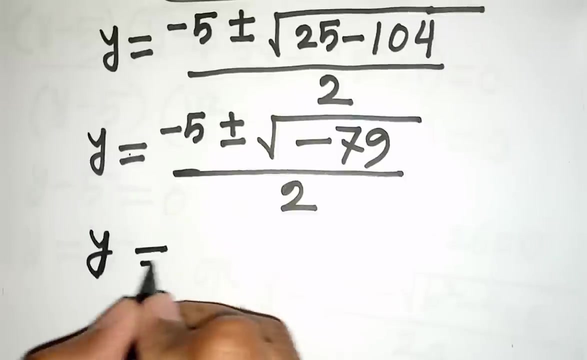 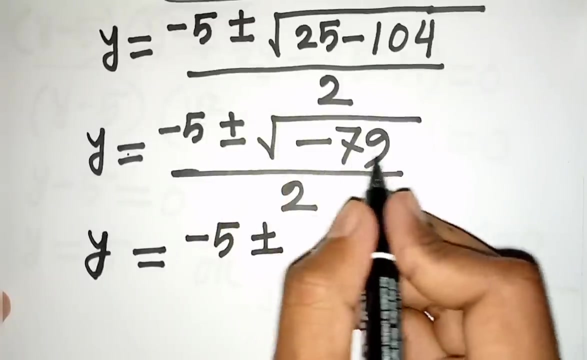 y is equal to minus 5 plus or minus a square root of 25 minus 104. that means minus 79 divided by 2.. Now we can write here: y is equal to minus 5 plus or minus. a square root of minus 79 is same as. 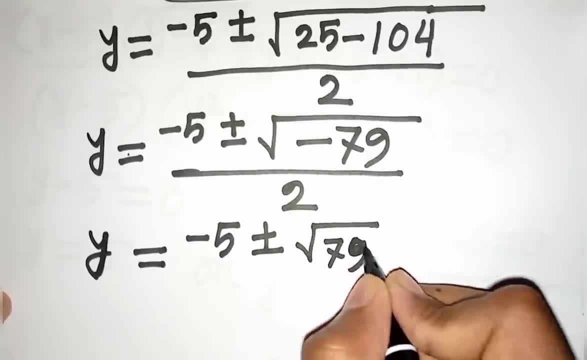 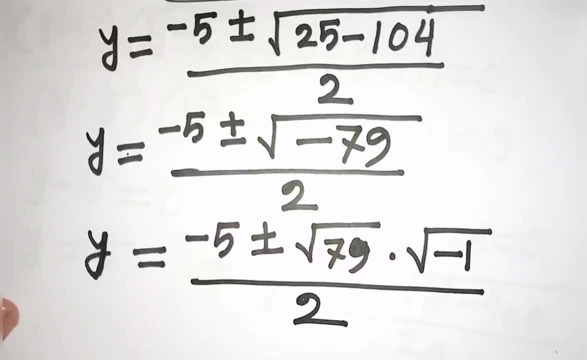 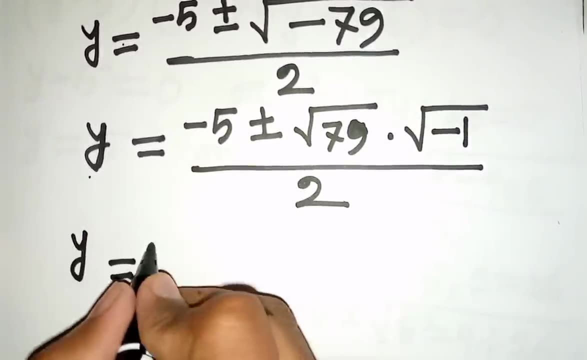 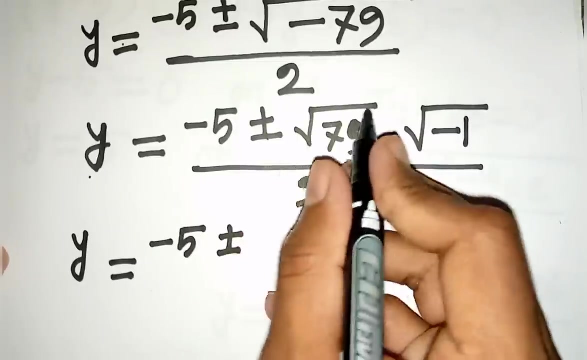 a square root of 79 times a square root of minus 1 divided by 2.. Now we can write here: y is equal to minus 5 plus or minus. a square root of minus 79 is equal to minus 5 plus or minus. a square root of 79 times a square root of minus 1. 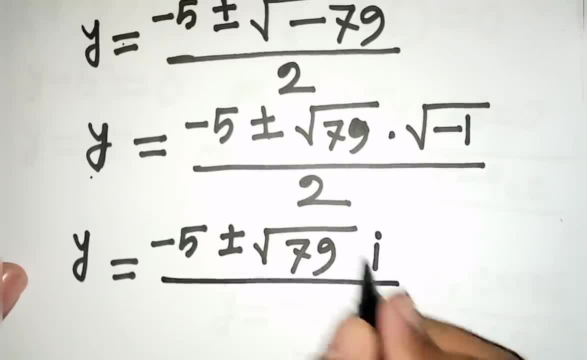 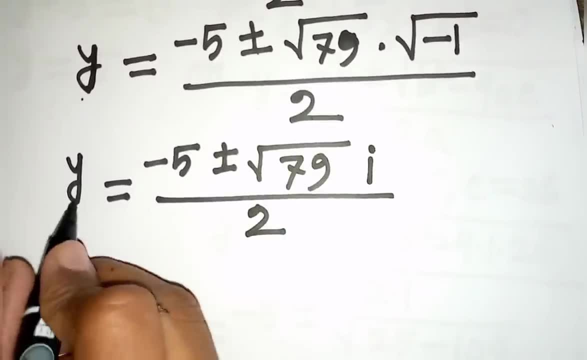 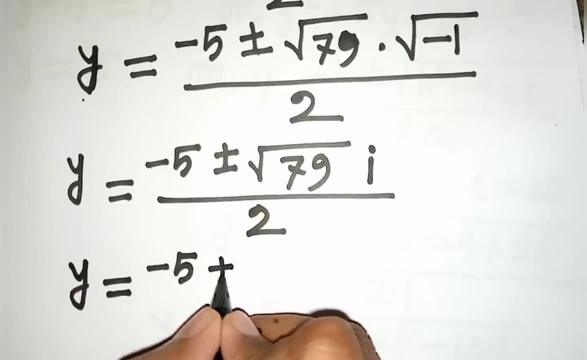 is same as imaginary divided by 2.. Now we see here two cases. so we can write here: y is equal to minus 5 divided by 2.. Now we can write here: y is equal to minus 5 plus a square root of 79, a square root of 79. 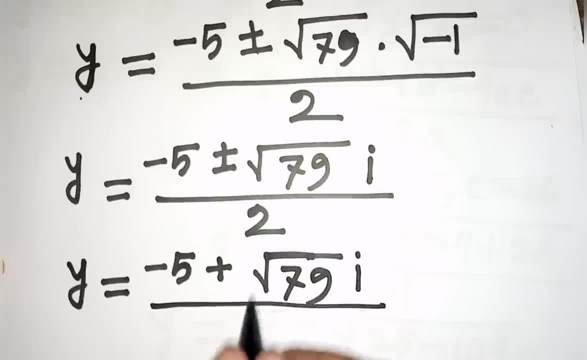 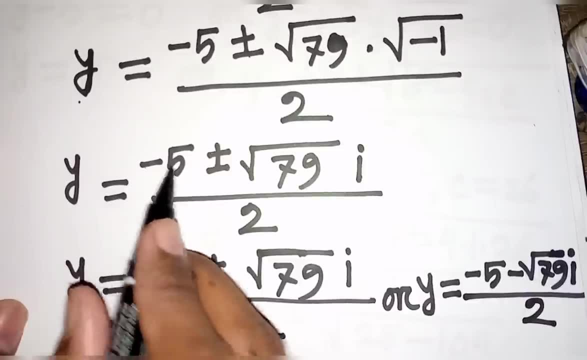 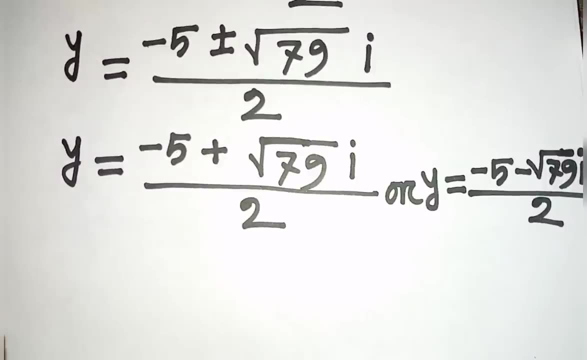 imaginary divided by 2 or y is. so y is equal to minus 5, minus a square root of 79 imaginary divided by 2.. So this value and this value are not equal, These are not accepted, so these are rejected, because these are imaginary values. so our 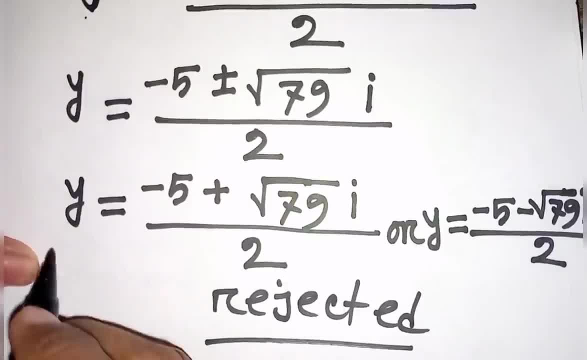 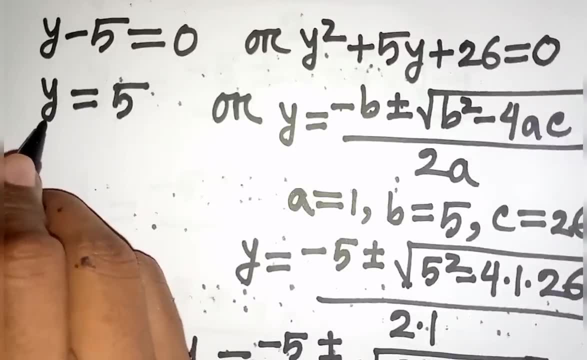 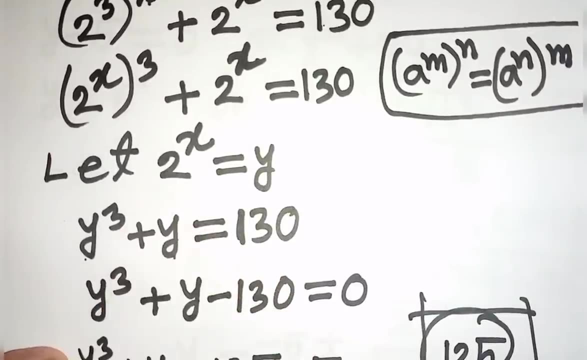 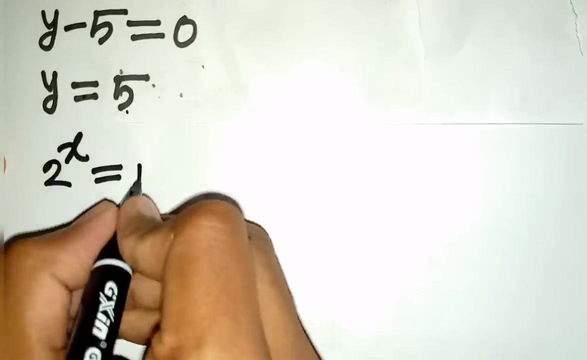 real value will be. so real value of y will be: y is equal to 5. but remember: y, that means let 2 power x is substituted by y, so y. that means 2 power x. So y. that means 2 power x. So y. that means 2 power x is equal to 5.. 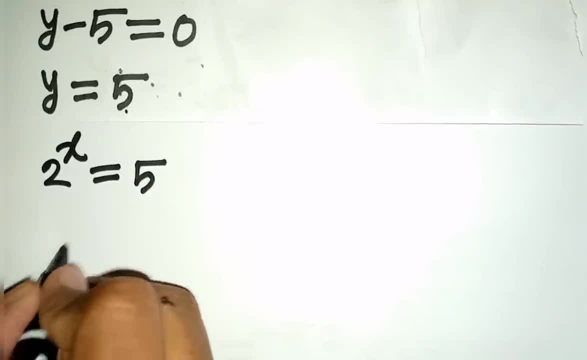 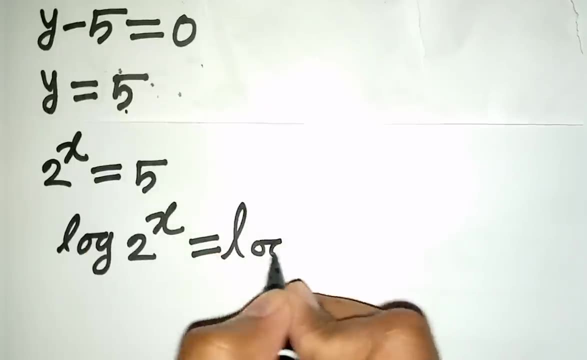 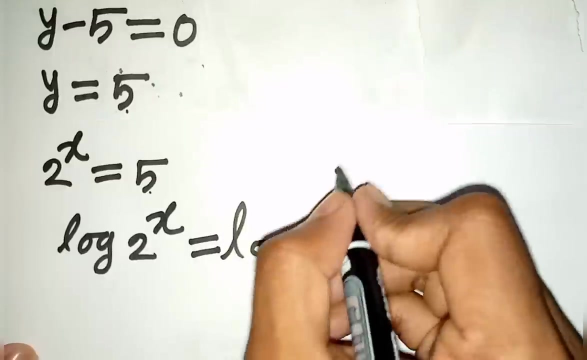 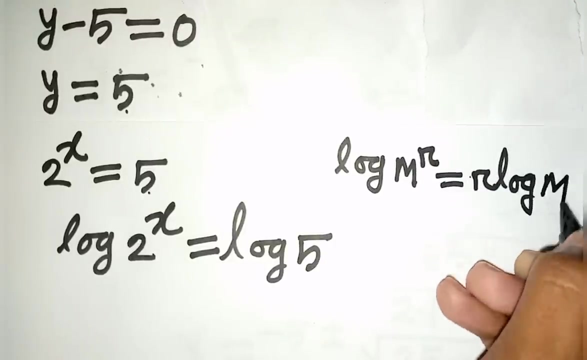 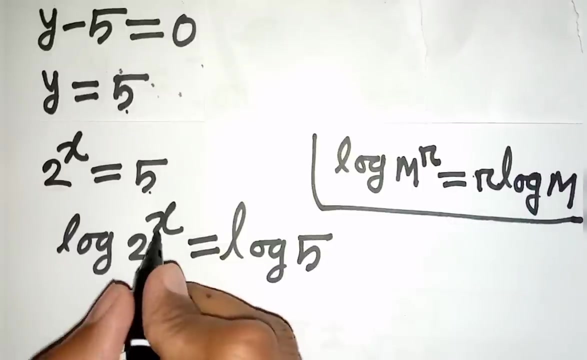 Now we take log both sides so we can write here: log 2, power x is equal to log 5.. Now here we can apply this formula: log m, power r is equal to r log m. That means this power move to here. so according to this formula, we can write here: x, log 2 is. 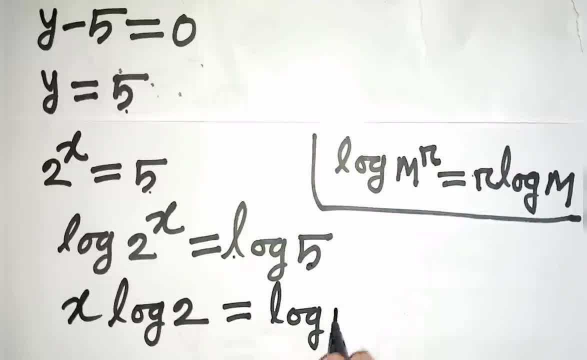 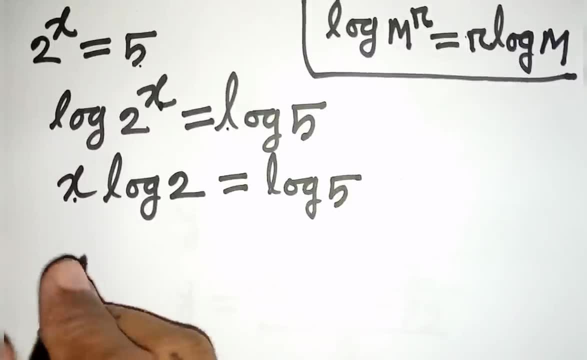 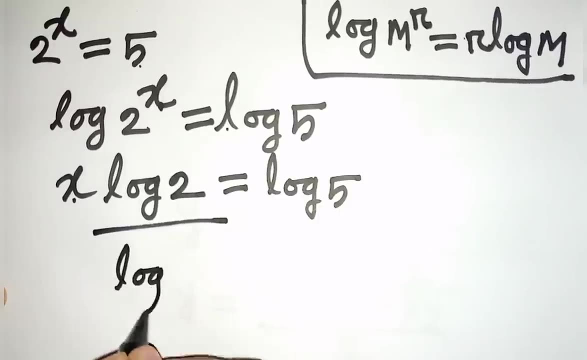 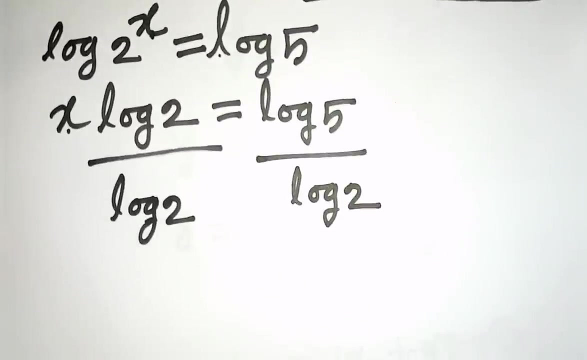 equal to log 5. log 5, that means this power move to here. Now we can write: here we need the value of x. so we divided by log 2, both sides, so divided by log 2.. Now we see this log 2. this log 2 will be cancelled. so here x is equal to log 5 divided by log 2.. 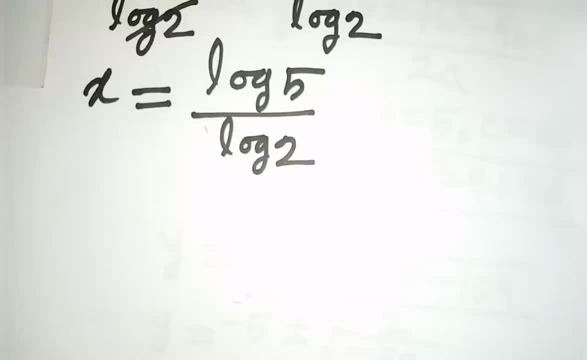 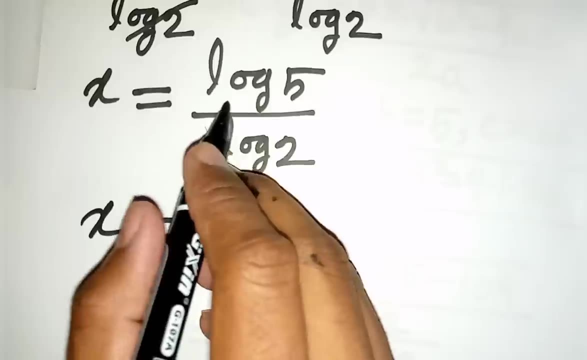 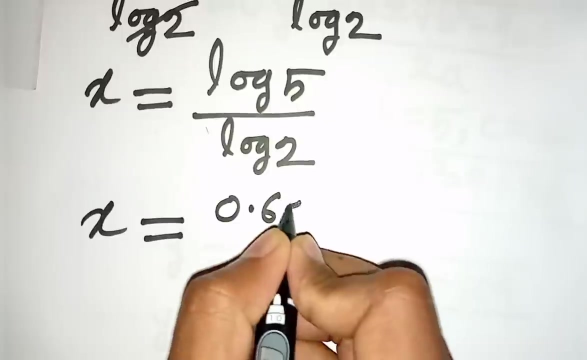 Now we can write here: x is equal to here. we use 2 power here. we can write here: y is equal to 2.. we use calculator. So the approximate value of log 5 is 0.699 divided by log 2.. The approximate 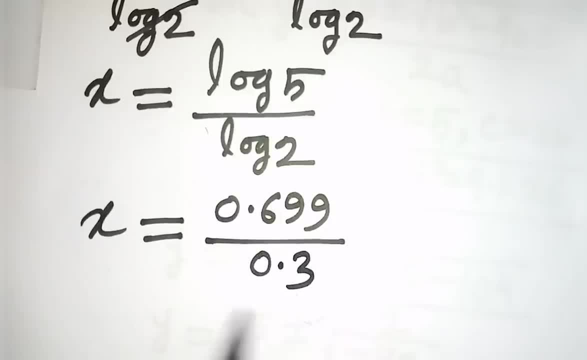 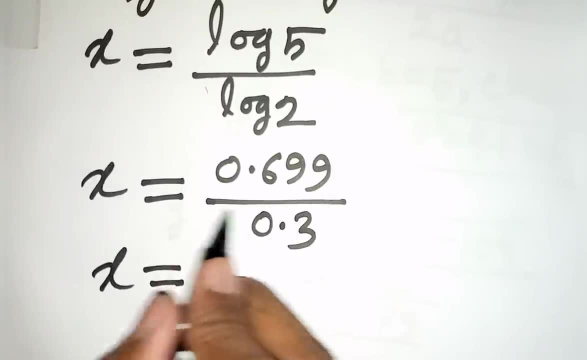 value of log 2 is 0.3.. Now we can write here: x is equal to 0.699. divided by 0.3 is 2.33.. So this is the approximate value of x. So x is equal to 2.33.. 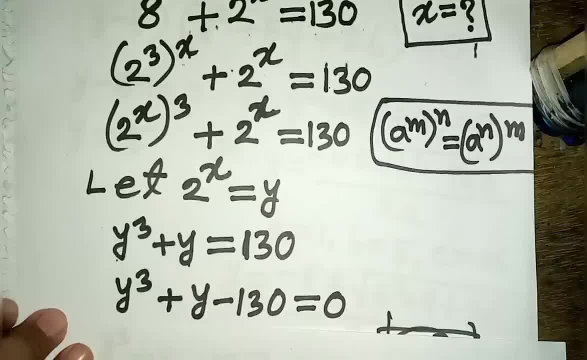 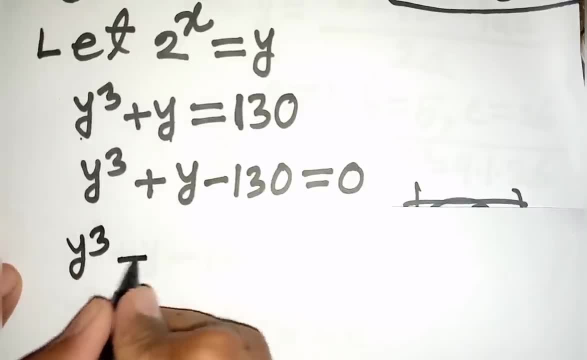 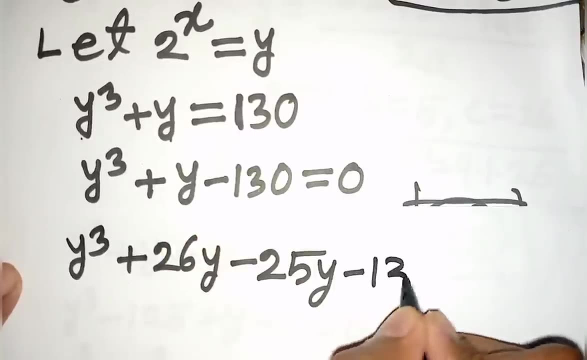 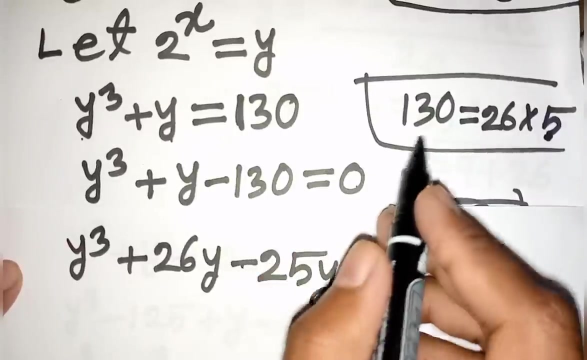 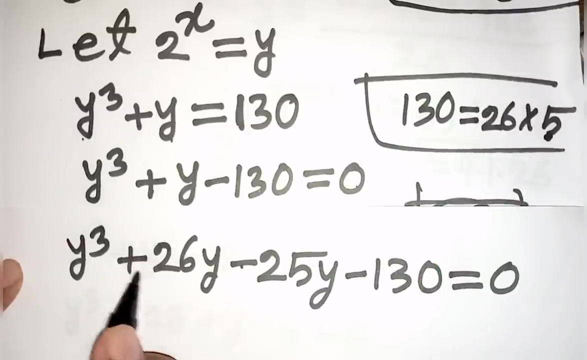 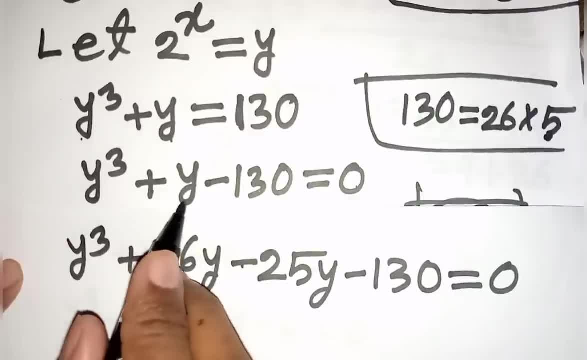 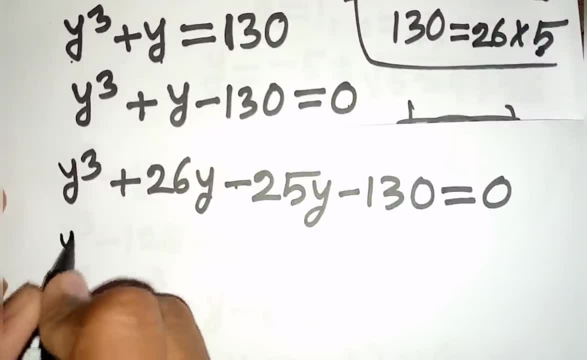 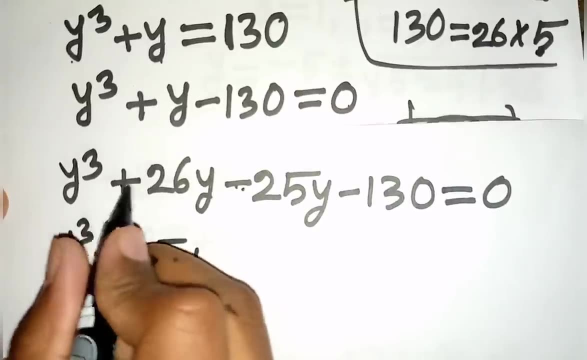 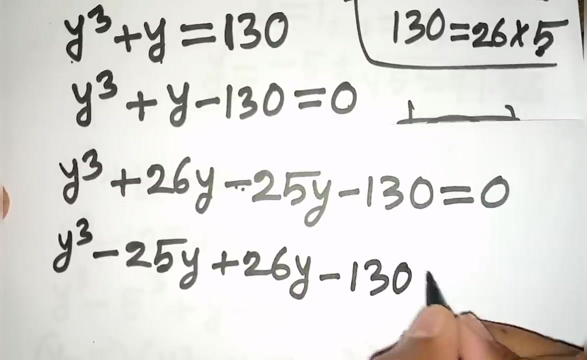 write here: y cube minus 25 y, That means plus y, Then minus 130 is equal to 0.. Now we can write here: y cube minus 25 y, Then plus 26 y minus 130 is equal to 0.. Now here we take common. 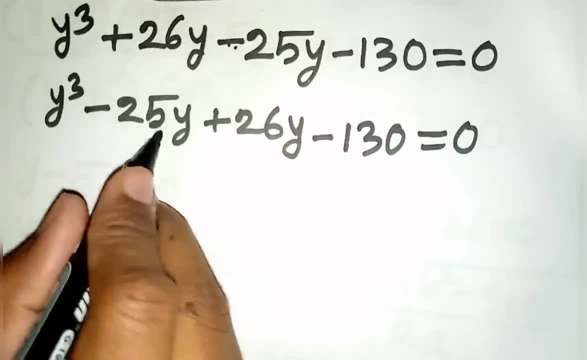 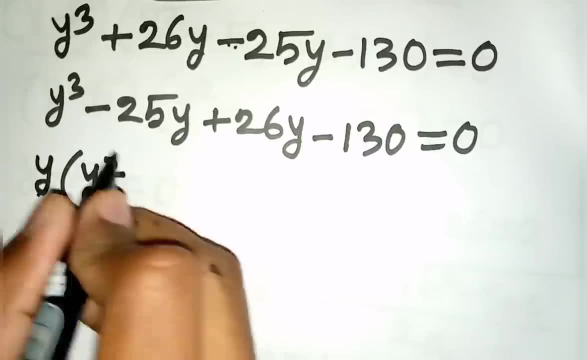 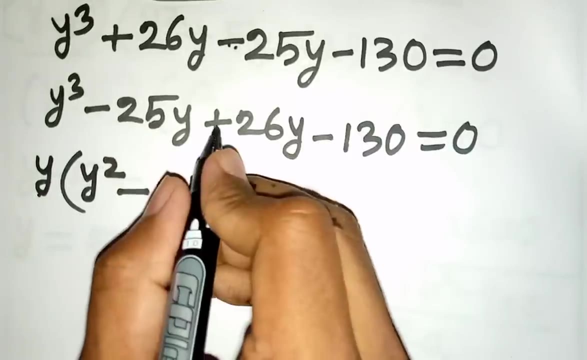 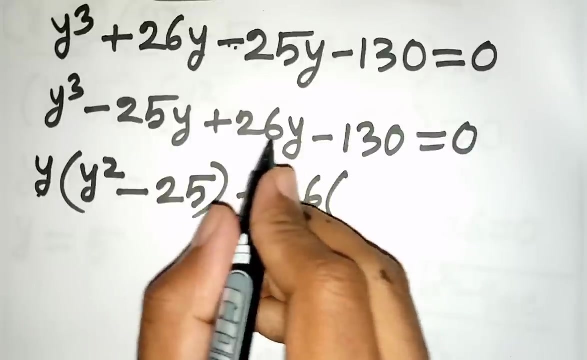 y, So y is out of the bracket. This divided by this, That means y square minus. this divided by this, That means 25.. Then here plus 26 is common. So plus 26 is out of this bracket. So this divided. 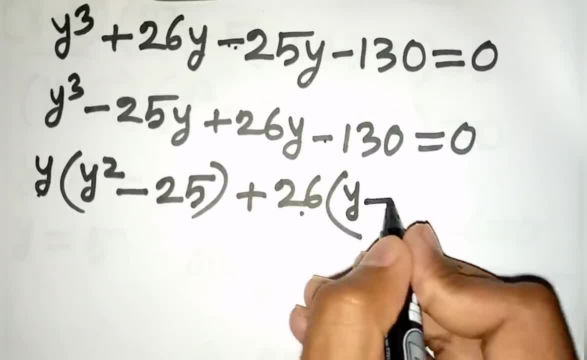 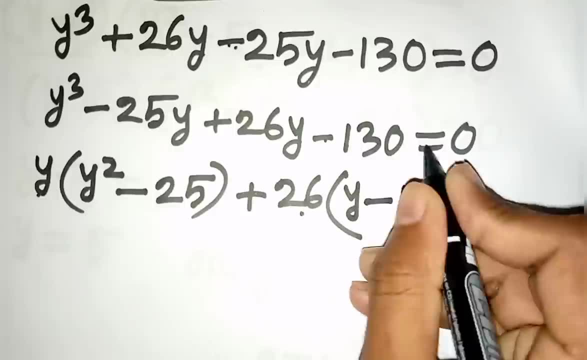 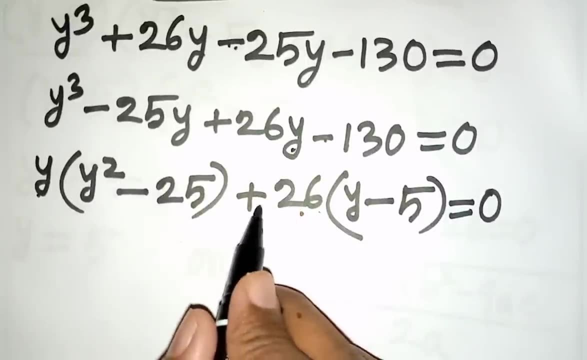 by this. That means y minus 130 divided by 26. That means 5 is equal to 0.. So plus 26 y divided by plus 26. That means y. Then minus 130 divided by plus 26. That means minus 5 is equal to 0.. Now we can write here y times y. 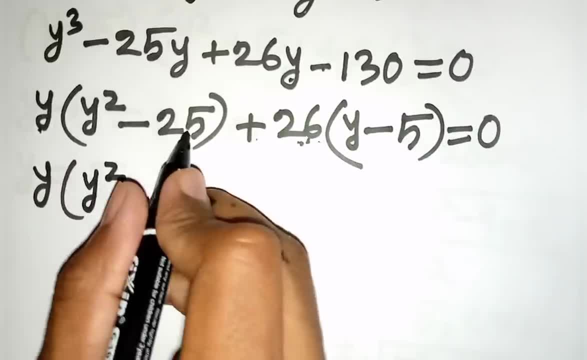 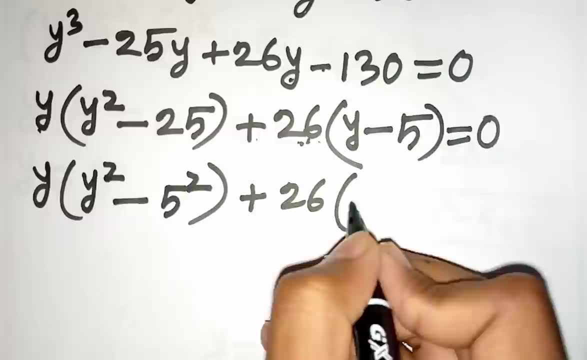 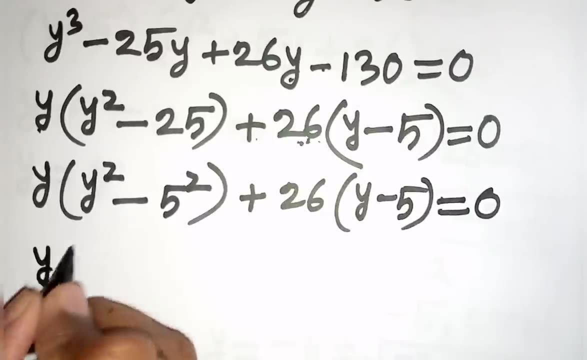 square minus 25.. Then plus 26 times y minus 5 is equal to 0.. Now we can write here y times. Here we can apply the formula of a square minus b square: Here a is s, y, b is s 5.. So according to formula, we can write: 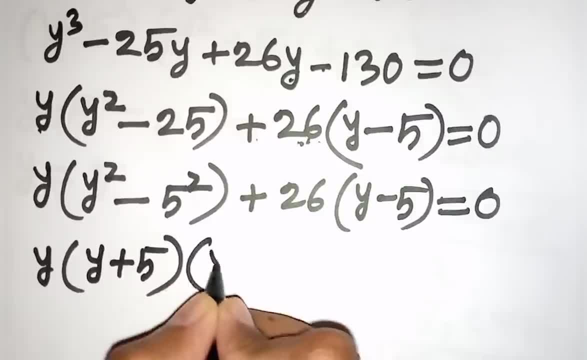 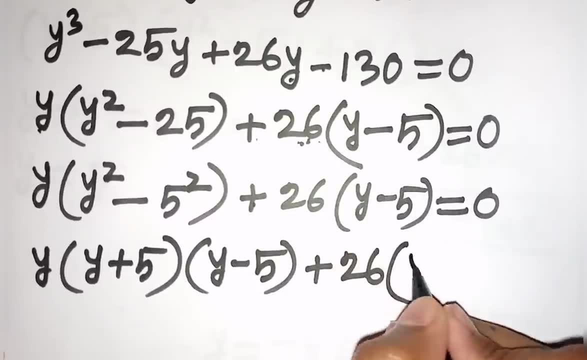 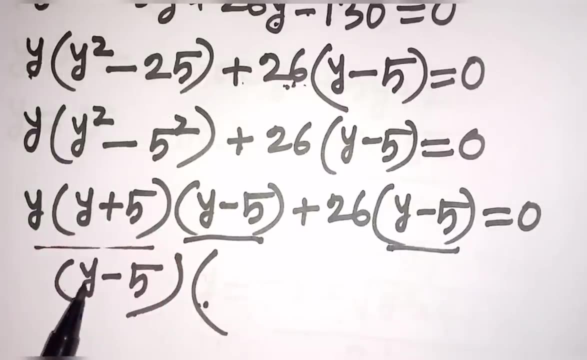 here: y plus 5 times y minus 5. Then plus 26 times y minus 5 is equal to 0.. Now we can write here: y times y minus 5.. Then plus 26 times y minus 5 is equal to 0.. Now we see y minus 5. y minus 5 is common, So bracket. 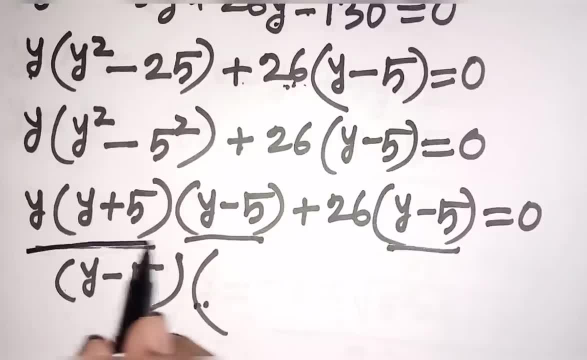 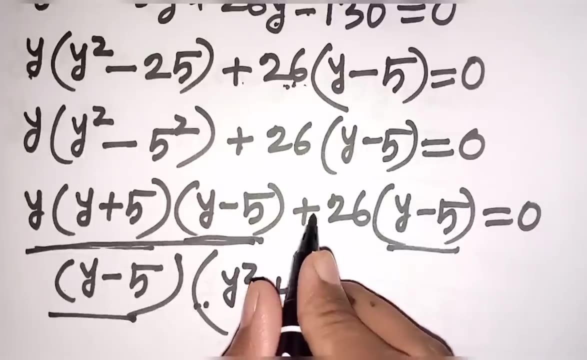 y minus 5 is out of this bracket. So this divided by this, That means y times y plus 5.. So y times y, It will be y square Y times plus 5.. It will be plus 5 y Then plus 26 times y minus 5.. That. 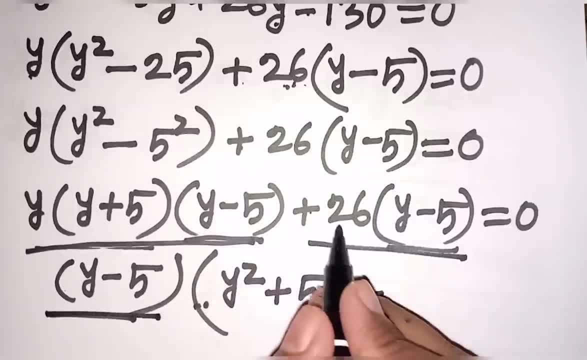 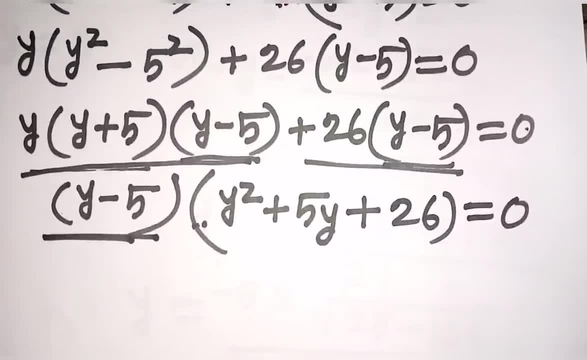 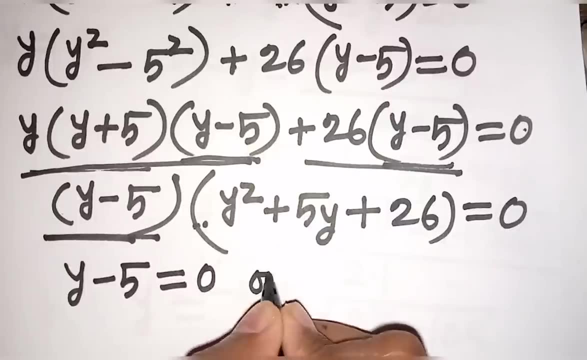 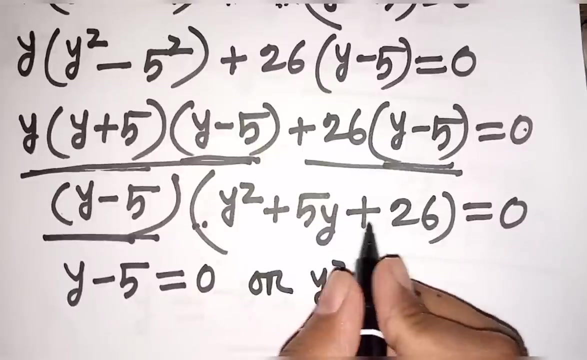 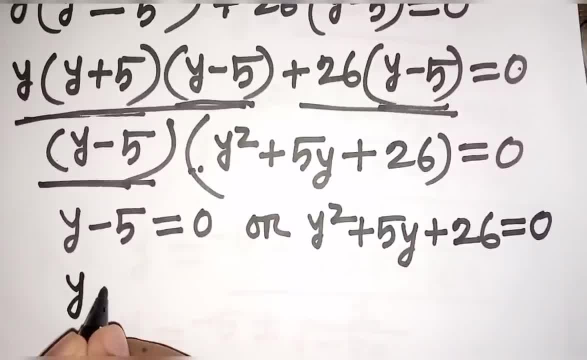 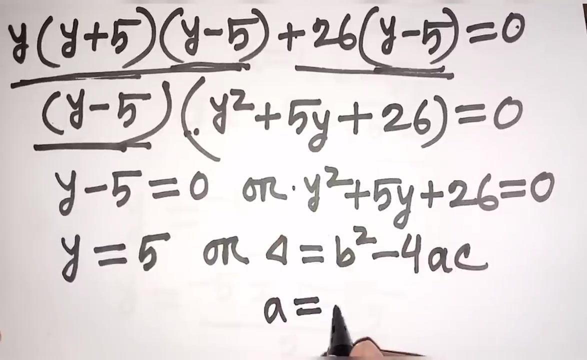 y minus 5 is equal to 0.. Or y square plus 5, y Then plus 26 is equal to 0.. Now we can write here: y minus 5 is equal to 0.. Now we can write here: y is equal to minus 5.. Take to the right side, So this will be plus 5.. Or here we can apply discriminant formula: delta is equal to b square minus 4 ac. Now here a is as on, b is as 5.. 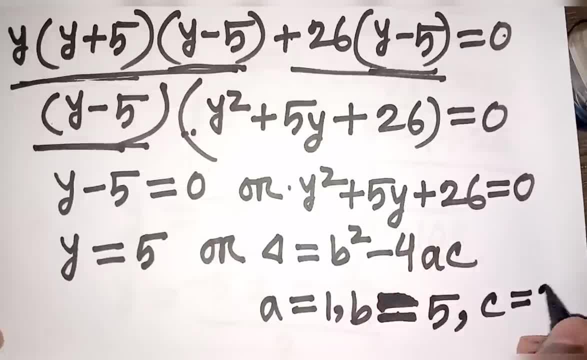 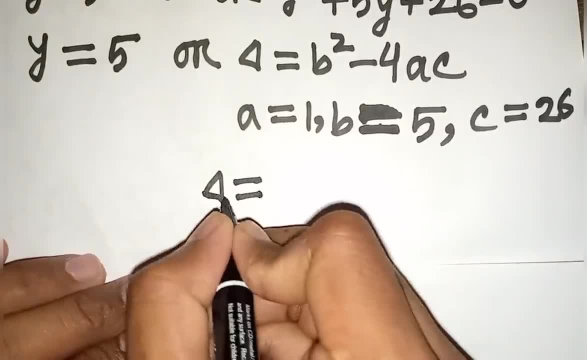 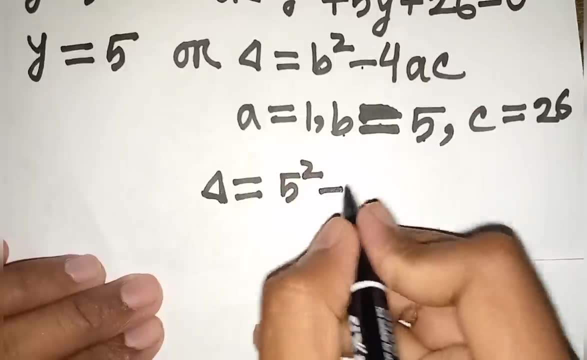 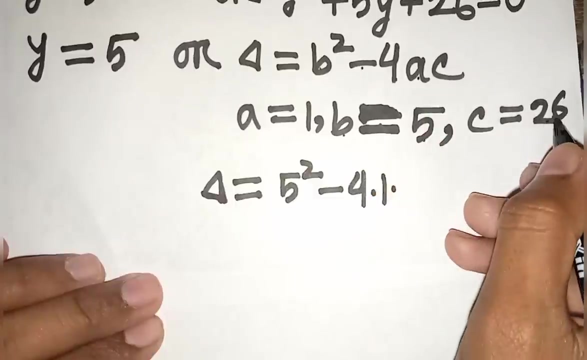 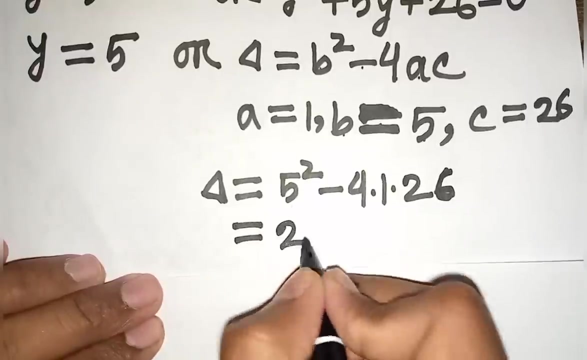 c is as 26.. Now so we can write here: delta is equal to b square. that means 5 square minus 4 times a. that means: on times c. that means: 26 is equal to 5 square. that means 25 minus 4 times on times 26. that means: 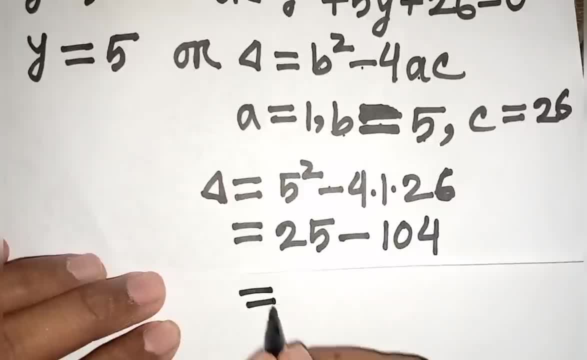 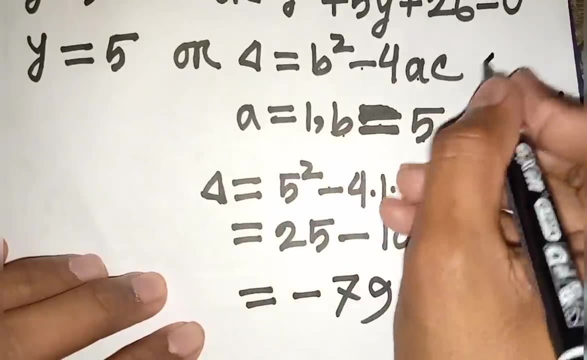 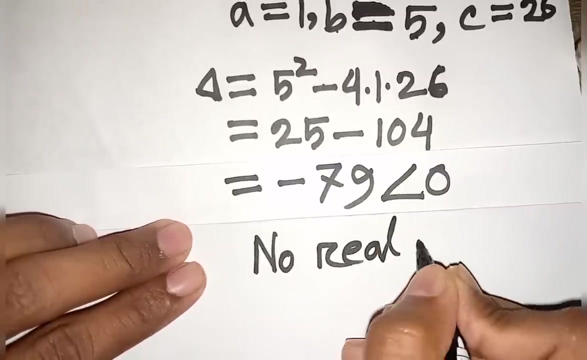 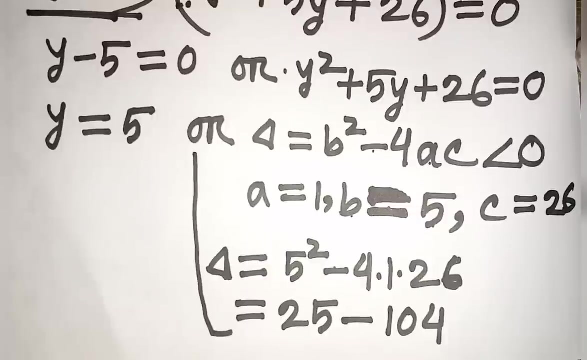 104 is equal to 25. minus 104 that means minus 79. so minus 79 is less than zero. So b square minus 4 ac is less than 0.. So b square minus 4 ac is less than 0.. So here no real solution. Now the real value of y will be: y is equal to 5.. But remember: 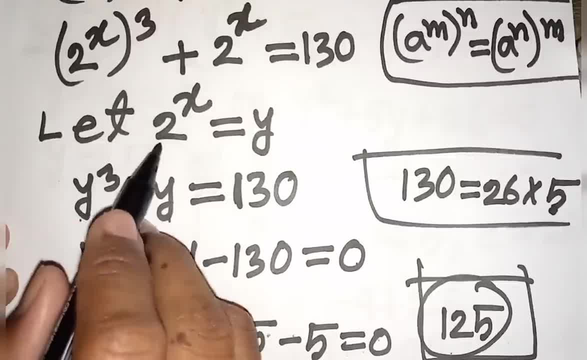 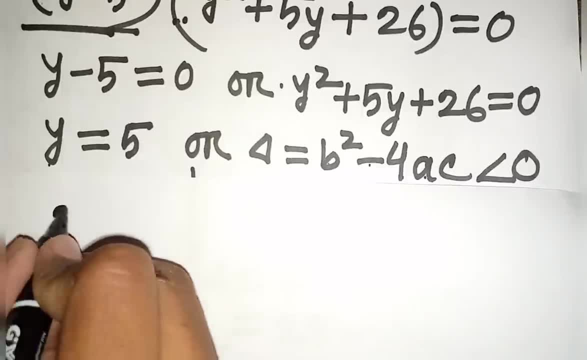 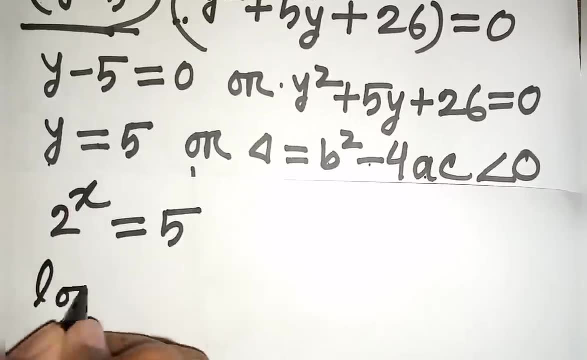 y, that means let 2 power x is substituted by y, So y that means 2 power x, So y, that means 2 power x is equal to 5.. Now we take log both sides, So log of 2 power x is equal. 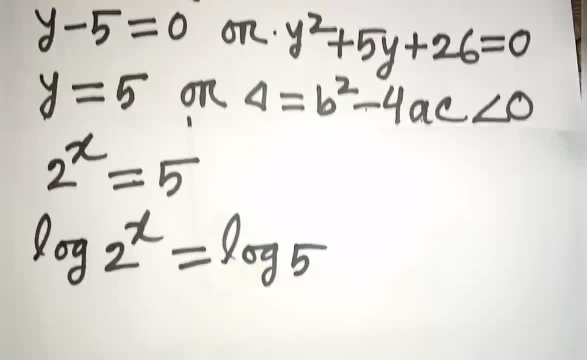 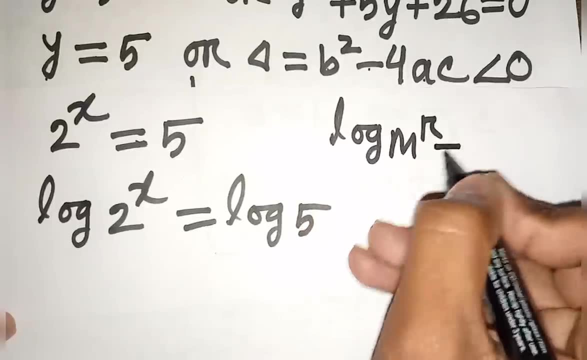 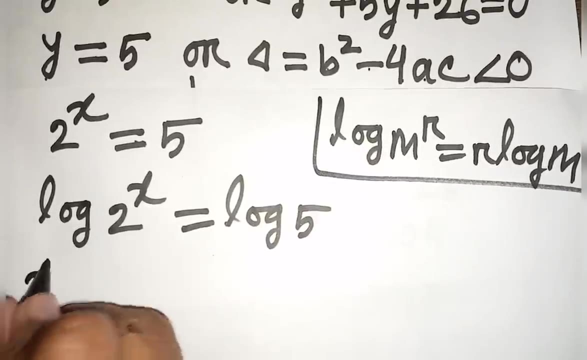 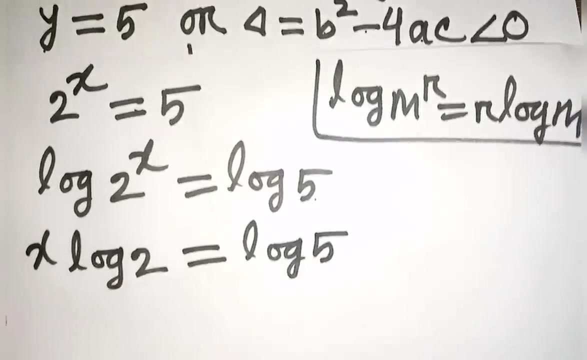 to log of 5.. Then here we can apply this formula: log m power r is equal to r log m. So according to this formula we can write here: x log 2 is equal to log 5.. Now we need the value of x. So we divided by log 2 both sides. So 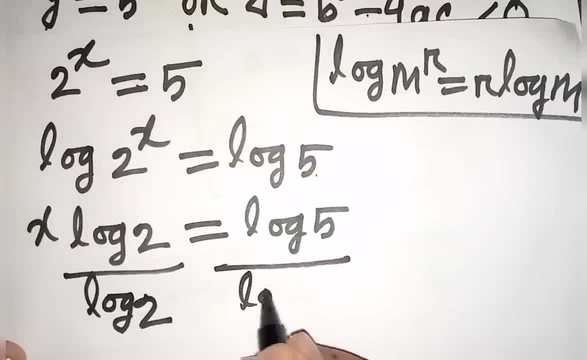 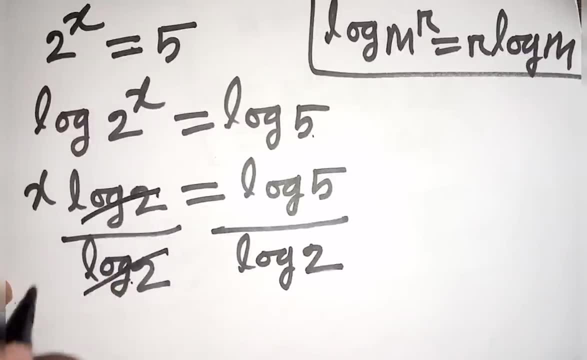 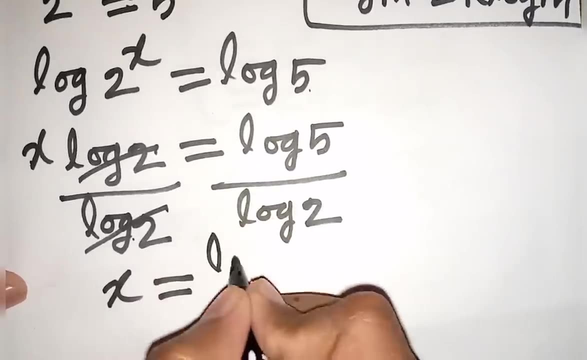 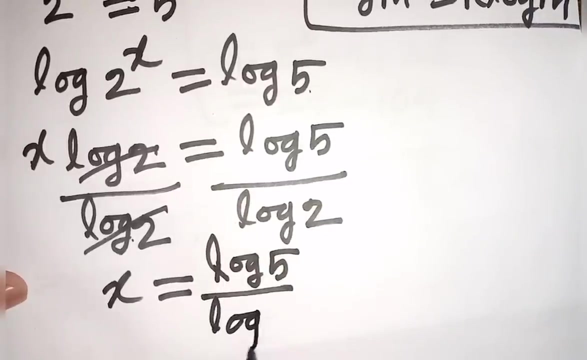 divided by log 2. divided by log 2.. Now we see this log 2. this log 2 will be cancelled. So here x is equal to log 5.. Now x is equal to log 5 divided by log 2.. So here we can write this log: x is equal to. 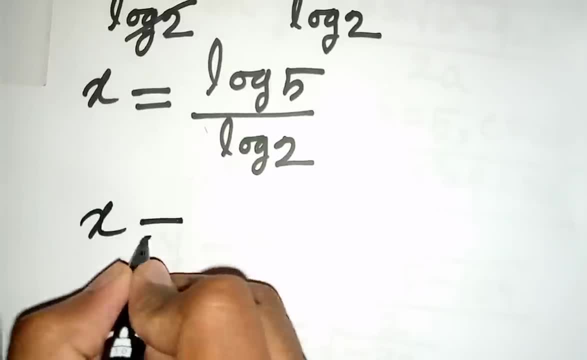 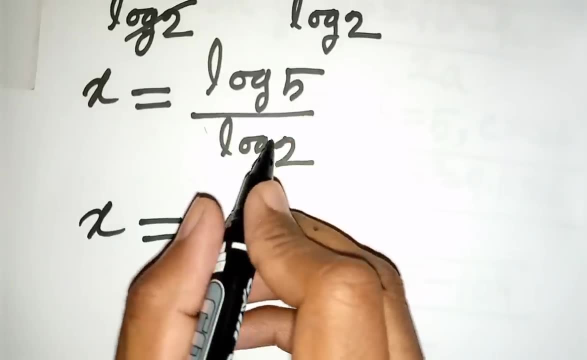 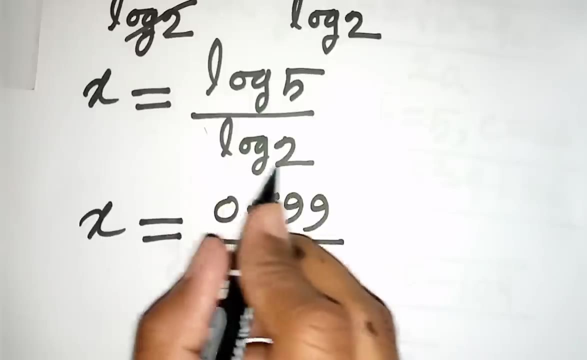 log 2 divided by log 2.. Now we can write: here x is equal to here we use calculator. So the approximate value of log 5 is 0.699 divided by log 2.. The approximate value of log 2 is 0.3.. 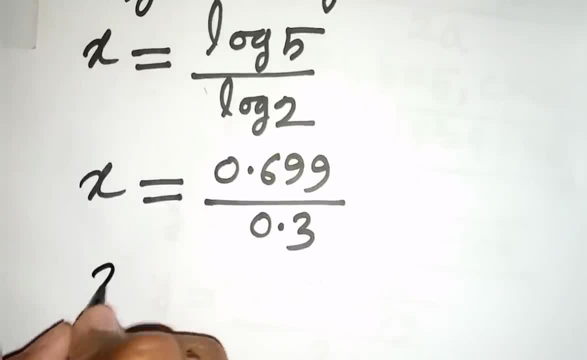 9.. Now we can write here: x is equal to 0.699. divided by 0.3 is 2.33.. So this is the approximate value of x. So x is equal to 0..